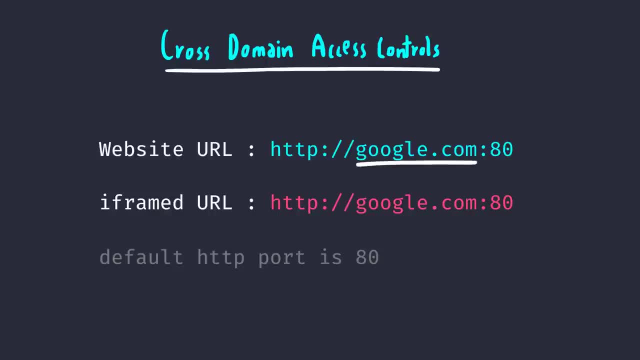 following three conditions are met: Firstly, same domain. Second, same schema. Thirdly, we have same port. These three things are the same between the iframe and the website. only then the browser lets you read cross domain data. This does not just apply to frames, but it also applies. 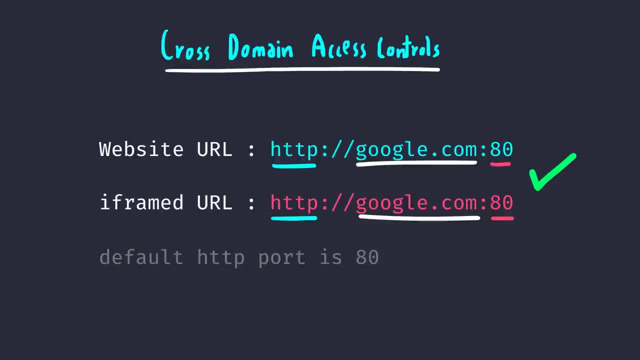 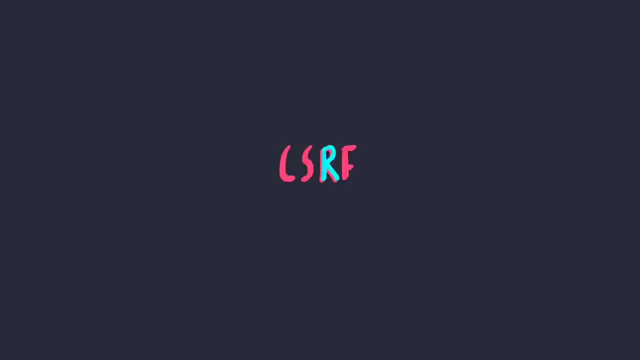 to other things like AJAX requests. Now that you know a bit about the fundamentals, let's continue our journey with CSRF attacks. First off, CSRF stands for Cross Site Request Forgery. This means one domain is making, or more accurately, forging, requests to another in order to modify. 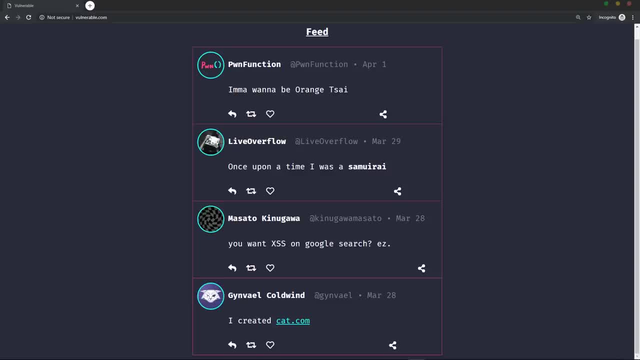 some value. For example, let's say we have a website called vulnerablecom and clicking on the delete button actually deletes our user account. Now we don't want to do that. And let's go and click on another link, which is catcom. Who doesn't like cats Best? 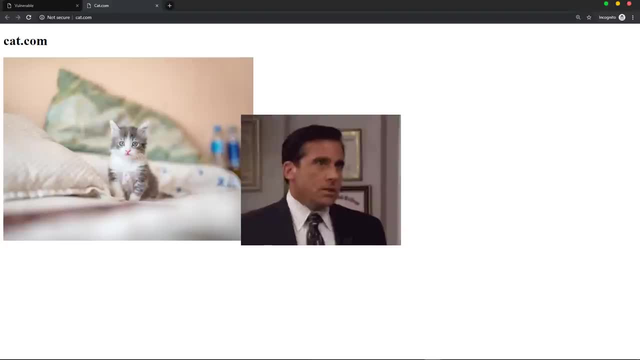 website in the world, right? No, you're wrong. In fact, this is the best website in the world. No, you're wrong. In fact, this is the best website in the world, right? No, you're wrong. 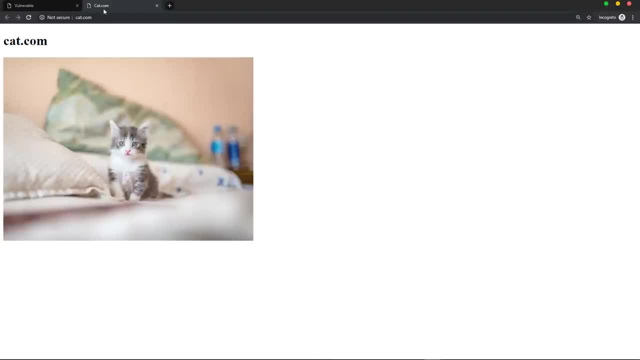 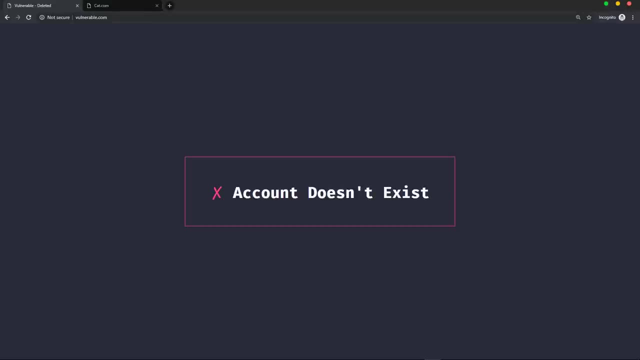 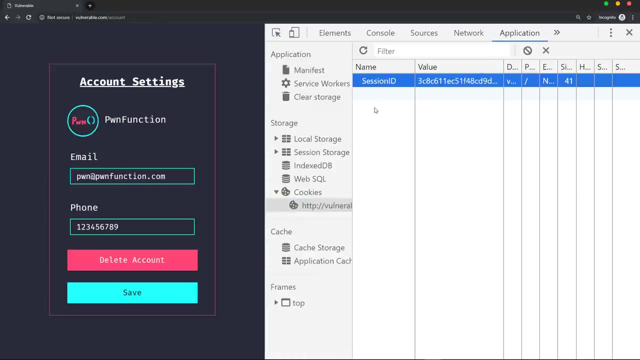 No, you're wrong. In fact, it just became your nightmare. It basically deleted your account on vulnerablecom just by visiting catcom. Let's break this down so that we can understand it a bit more. You've logged in to your account on vulnerablecom and you have some cookies saved in your browser. 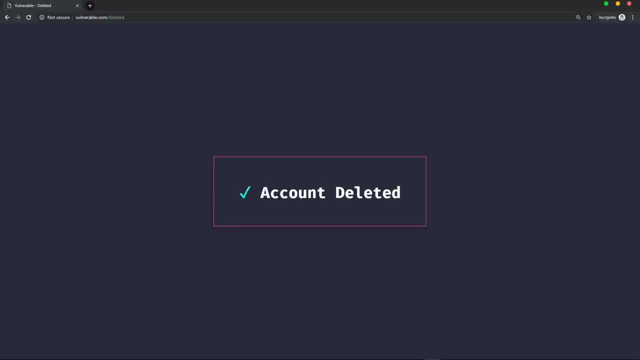 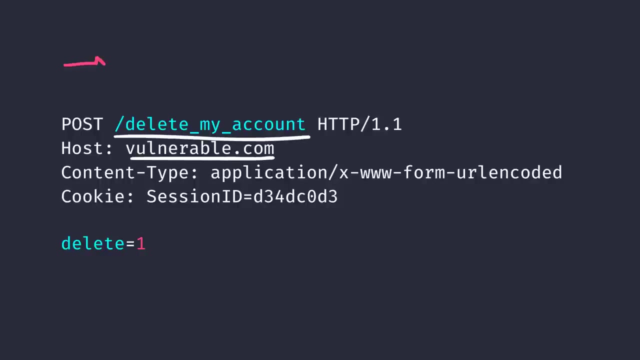 Same as usual. If you click on the delete button, it will send a delete request to this endpoint, vulnerablecom. slash delete my account, But when you visit catcom there was a request made. But when you visit catcom there was a request made to the exact same endpoint, vulnerablecom. 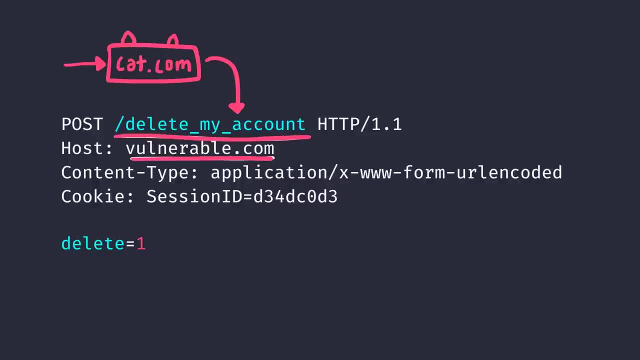 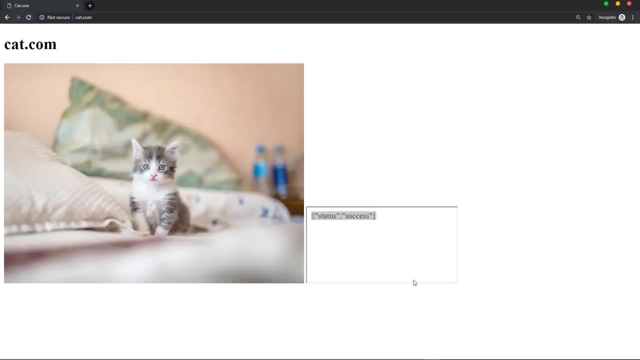 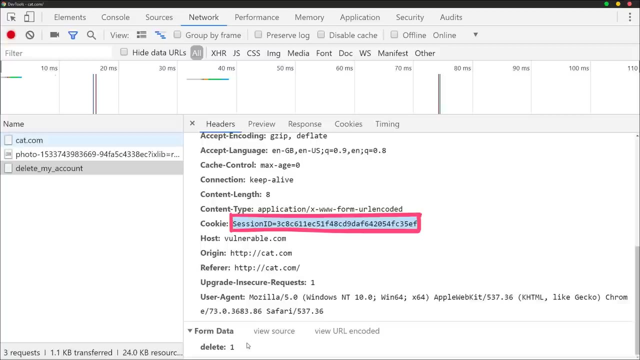 slash, delete my account. But it was made from catcom. And now remember what I told you earlier: On every single request, the cookies are automatically sent to the website, regardless of your current domain, Unless there are some flags set to it which we're not going to talk about. 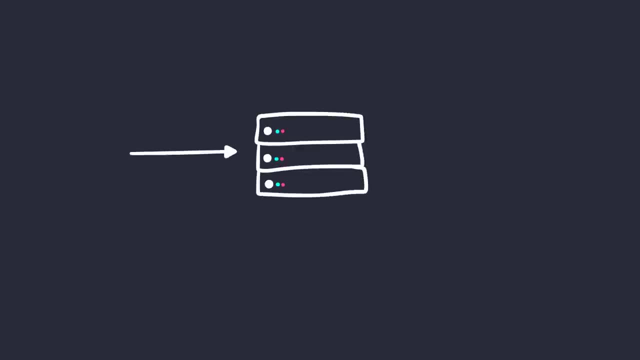 But anyways, this means that a delete action happens in the context of your session, Ultimately deleting your account forever. So, in short, catcom forged a delete request to the vulnerablecom. This is CSRF or Cross Site Request Forgery. This is an old vulnerability. 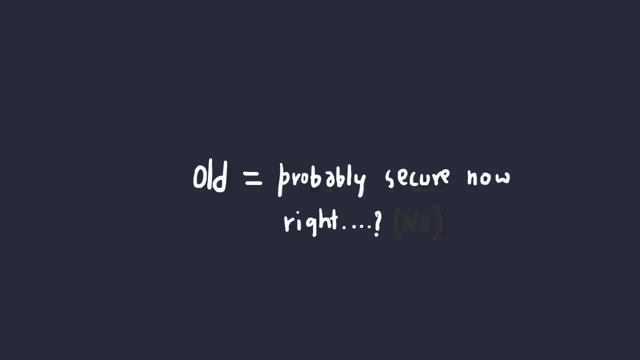 It's been here for a very long time And there are proper protections against this, And one popular and widely accepted solution is by using randomized tokens, which are also called as anti-CSRF tokens. This will be generated randomly by the web application in the backend and sent to the 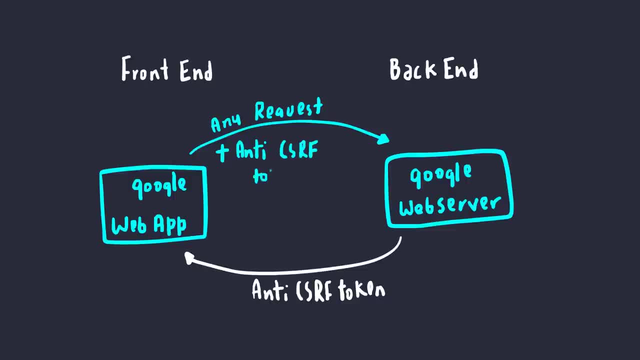 website. On every request, it's validated, so that the other website can't make cross origin requests or cross domain requests because of the fact that it doesn't have any knowledge about this new token. Earlier, I also talked a bit about same origin policy. 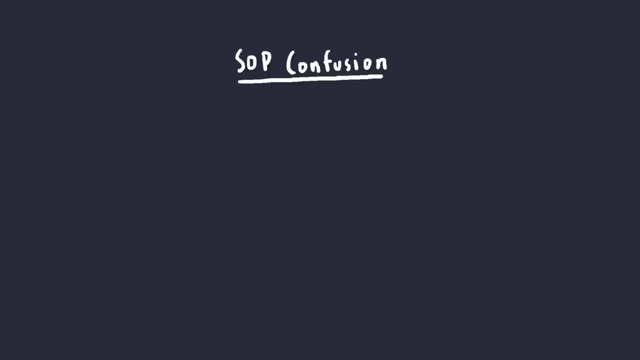 The reason for this is because I wanted to make a point clear By doing CSRF. There is no same origin policy bypasses, Which means we're simply making requests to other websites, which are totally allowed, but we can't read the responses, which is basically blocked by same origin policy. 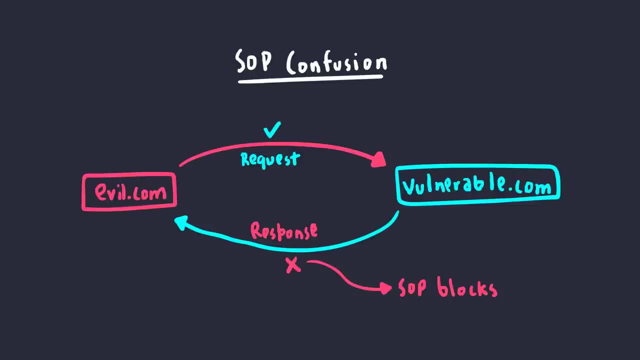 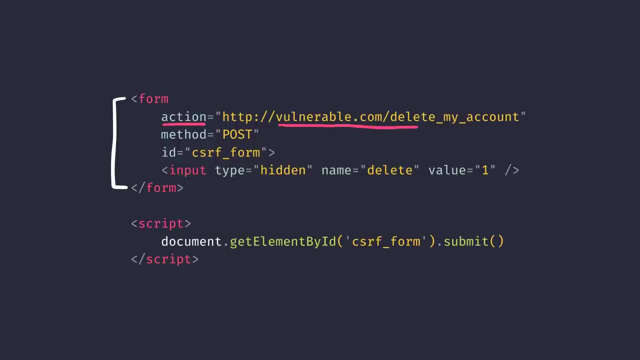 But again, no rules of same origin policy is broken. Now that we know the idea behind this attack, we can take a look at the code behind catcom to understand everything a bit more. As you can see, we have a form And the action of this form is set to delete endpoint of the vulnerable application. 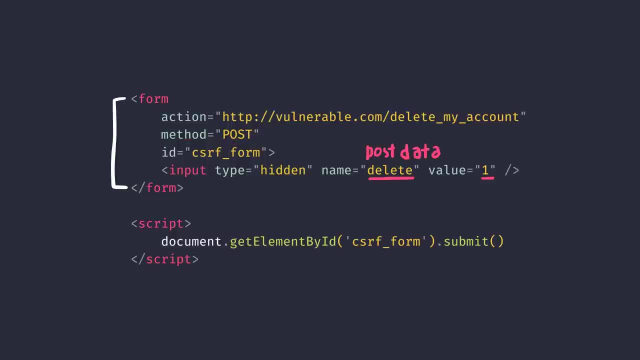 And the method is set to post. One additional thing that you can see is that there's some JavaScript which submits the form automatically, so that there's no user interaction or whatsoever. In addition, instead of form submissions, you can also use JavaScript to make Ajax requests. 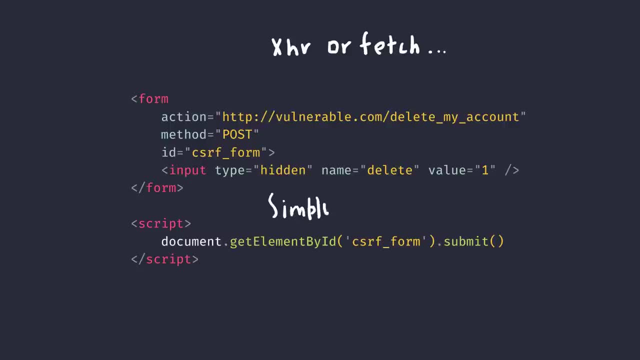 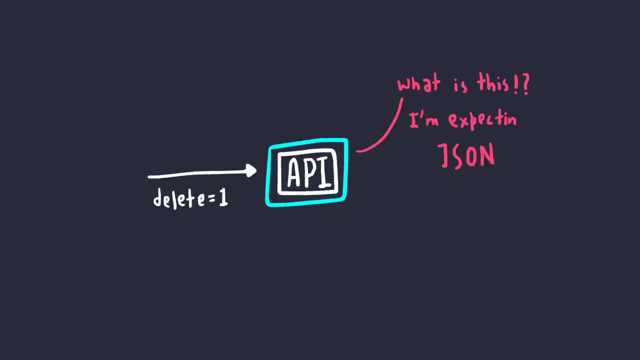 in the background, so everything happens asynchronously. Simple, but not always. Sometimes the web server will be expecting some JSON value, because we see a lot of APIs these days And it's very common for you to find CSRF with some JSON in it. As you know, in HTML the normal post request is going to be through a form. 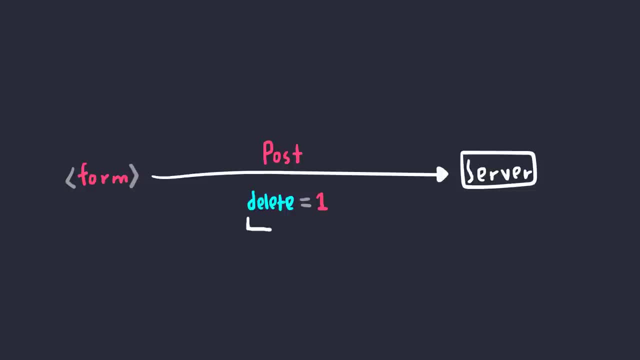 And usually post data when it comes through a form, has the generic key value pair but not JSON. If you think about how these post parameters are created from the HTML elements, you can actually figure a way around this. Suppose we had an endpoint called slash delete item, which takes a JSON, post data and deletes. 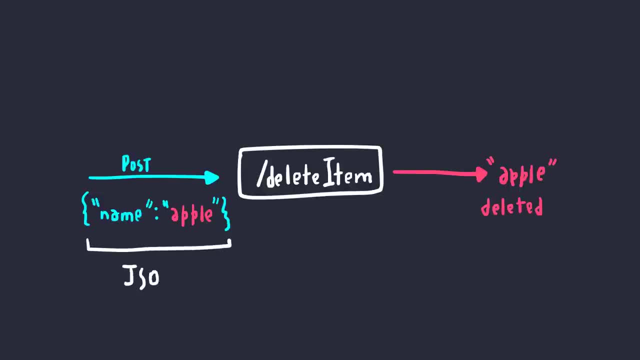 the specific item. As you can see, we have some JSON data here and we need to send it over to the website as a CSRF attack. But how can we send JSON data using forms, Because form submissions are not JSON stuff, right? 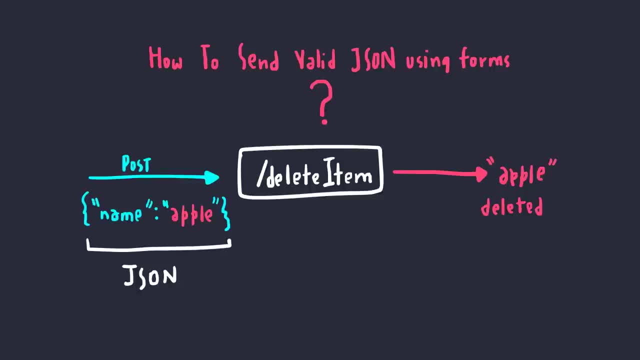 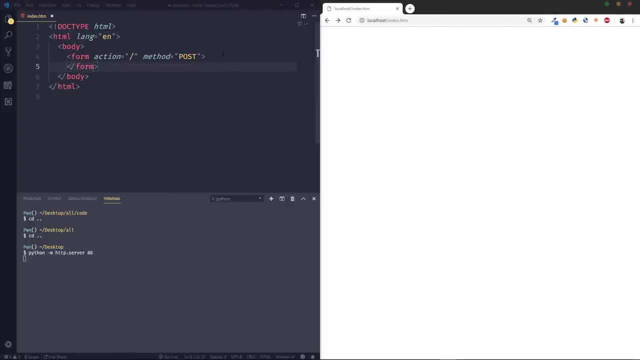 You can pause the video for a second and try to think about how you can do that. I'm going to show you how you can do that. Let's create a simple form to try this out. If we set the name of the item to something like Apple and send a request, we can see. 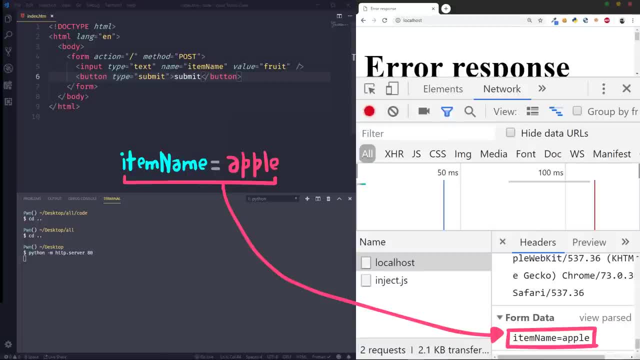 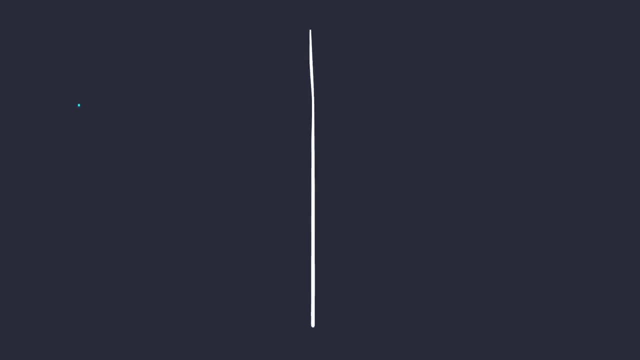 what's actually going on. As you can see, the majority of the string is controlled by the user, So let's try to craft something that looks like JSON. In the left, you can see the item name and the value, which is Apple, but we need something. 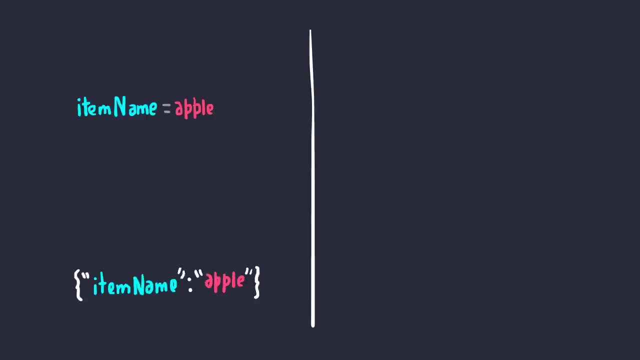 like this, a proper, valid JSON string. Now let's go step by step into creating from this to this. First off, we need some curly brackets. We can simply replace the item name to our JSON string. As you can see, we are already a lot closer. 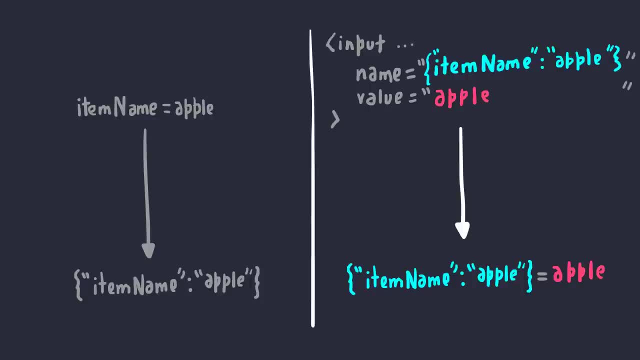 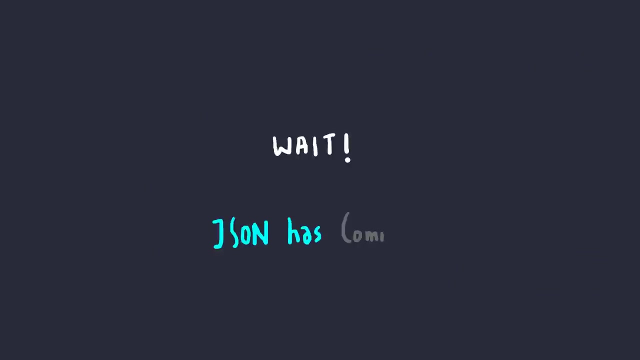 We have everything we need. but there's one more thing. It's not really a valid JSON data, As you can see, there's some text at the end which mean nothing. So, in order to get rid of this, You can make them as comments. but wait, JSON doesn't support comments, right? 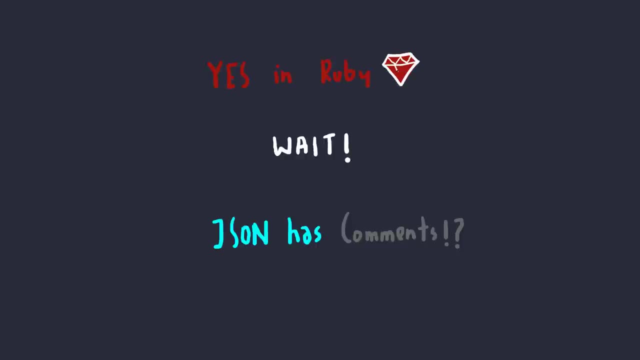 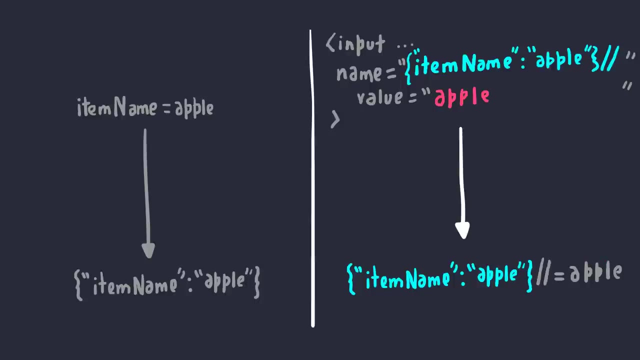 Well, it doesn't, but in Ruby it's actually a thing. Comments are kind of allowed, So you can simply add two forward slashes at the end and get this working. But hold on a minute. What if it was not Ruby? What if there was no JSON comments? 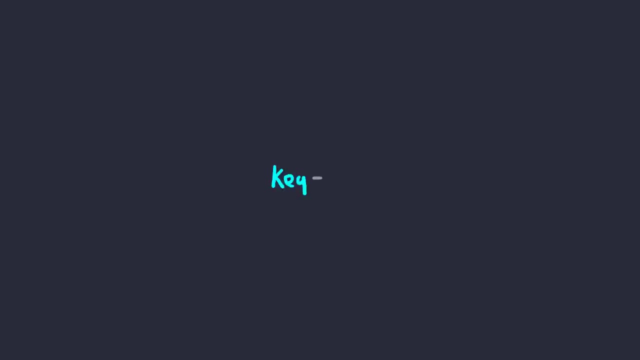 Well, we might have to think a bit differently. Since we also control what's after the equal sign, We can kind of make this work. We can simply add another key value pair in this JSON string, which doesn't mean anything. We can simply put it as junk and make this a valid JSON data. 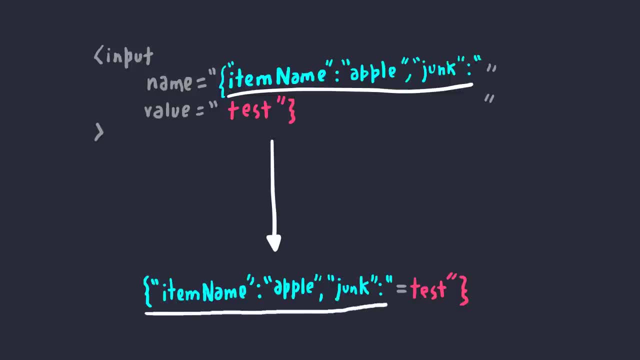 As you can see, this part is the first part, which is the name of the HTML element, And this part is the value. The equal to sign in the middle goes into the string equals test. Now, this entire thing is a valid JSON string. 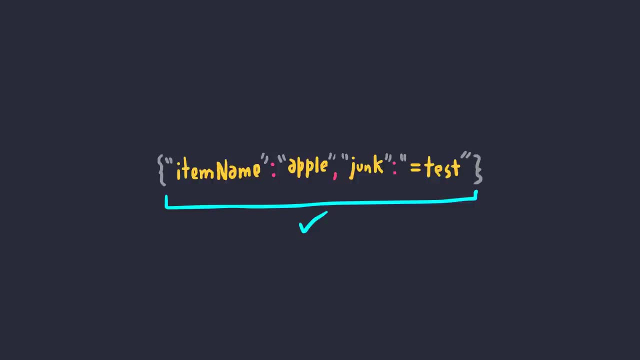 When this is passed, everything works. Only the item name is pulled out from this JSON object and the junk part is ignored. There we go. That's a simple way, But there's also another simpler way of doing this, and that is by using Ajax request. 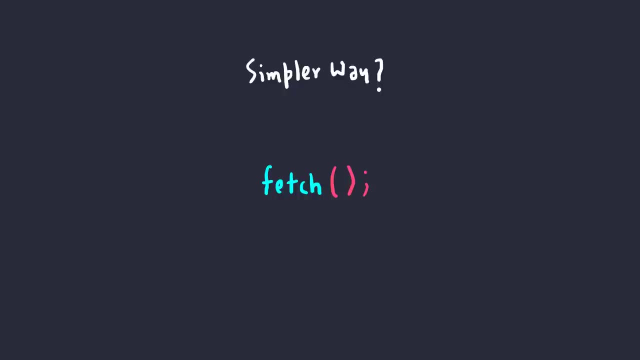 You can simply use fetch request and send the JSON string as the body. A lot simpler. I know, As usual we're going to get the same origin policy error, but we don't really care about this. We're just going to hit the server and our update action is going to happen regardless. 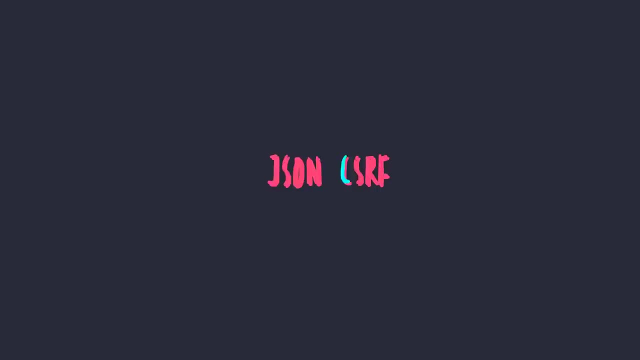 of the output. The form and the Ajax way that you just saw now only works if the content type header is ignored by the server. But many times you'll find yourself that these content type headers are actually required for this to work. Sometimes the web application might be expecting this. 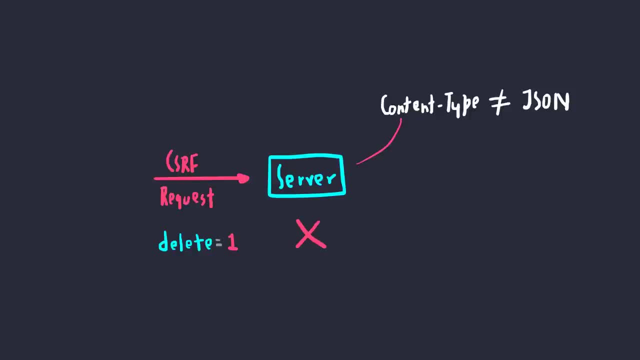 So we're just going to hit the server And we're going to use the same method. We're using a content type header being set to application JSON, which indicates explicitly that we're dealing with JSON data. Now the thing is, we can't just set another header in the form 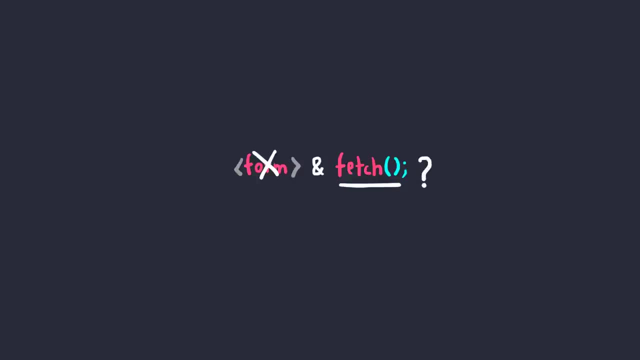 But we can set this in JavaScript, but there's still a problem. The browser doesn't just allow you to set any headers you want, unless the server explicitly lets you do it using CORS. Now, what is this? What is CORS? CORS stands for Cross-Original Server. 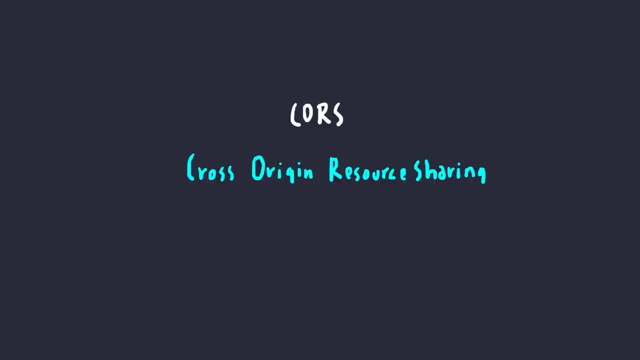 And what is CORS? CORS stands for Same-Origin Resource Sharing, And this is basically a bypass for Same-Origin Policy in a good way. of course, This is only allowed if the server explicitly lets you. This feature is quite useful than what you think it might be, because of the fact that 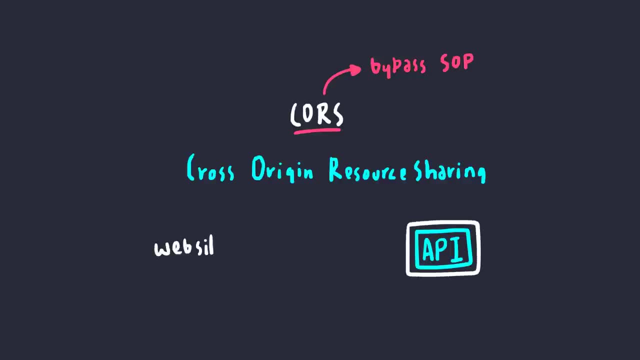 APIs are all over the place And usually APIs are going to be hosted in a different domain from the one that's actually making requests. In these kinds of situations, it's necessary to have a proper way to communicate. Coming back to this CORS thing, you can only set the content-type header if the server 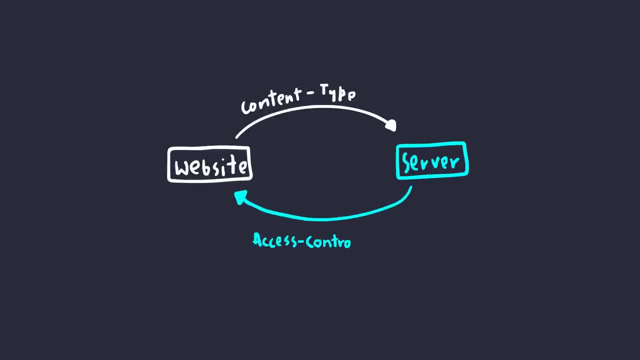 sends back your domain and the header that you want to set, which is content-type in the response header. To be specific, it's access-control-allow-origin and access-control-allow-headers. Only then it's possible for you to make JSON-CSRF requests with the content-type header being. 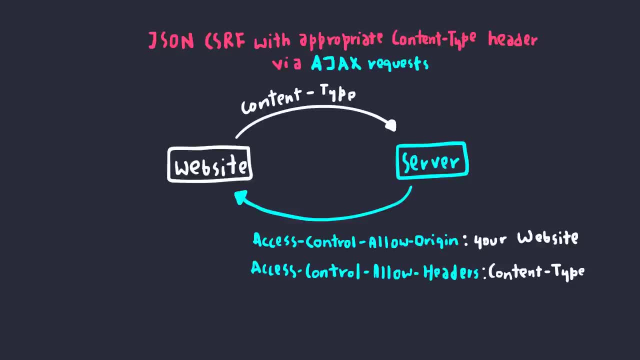 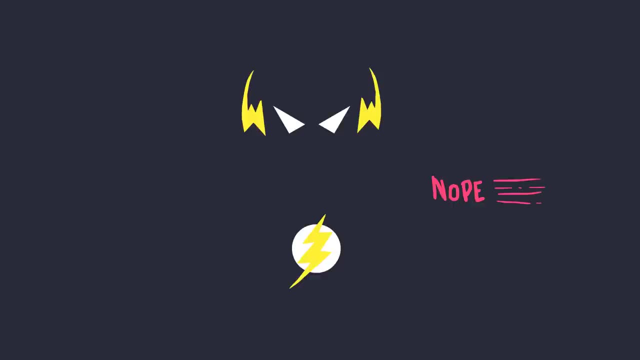 set to applicationjson. But there's another way of actually making this work without using any of these, And it's by using Flash. No, not the one from Justice League, but you know, if we had them it would have been a. 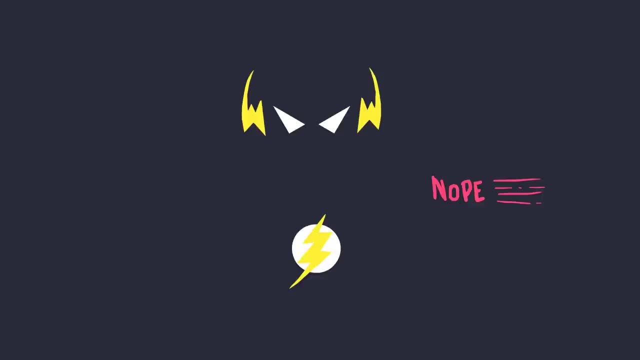 lot easier to hack stuff, if you know what I mean. Anyways, getting back to Flash, I mean the old Adobe Flash, Remember one of those? is that still a thing? I don't know. In about a year it's just going to completely vanish, pretty much. 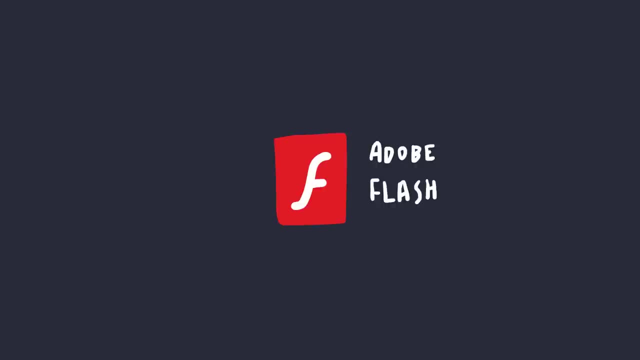 But yeah, Flash files, They can help you In this case. Flash files aren't directly affected by the same origin policy because they have their own thing And I'm not going to get into details. but you can look it up on Google and do your. 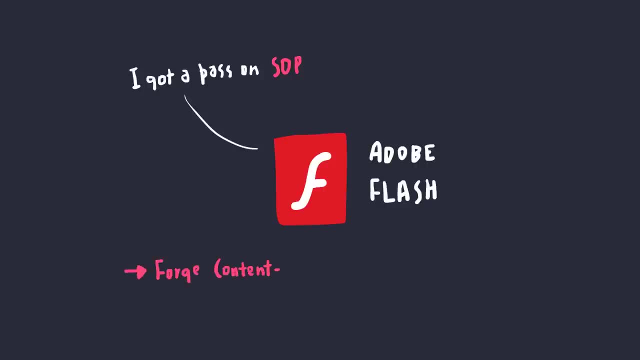 research, I guess. But again, you can forge the content-type header using Flash files. But the thing is, the cookie won't be sent along with it, Unless we have that cross-domain XML and other things which we're not going to talk about. 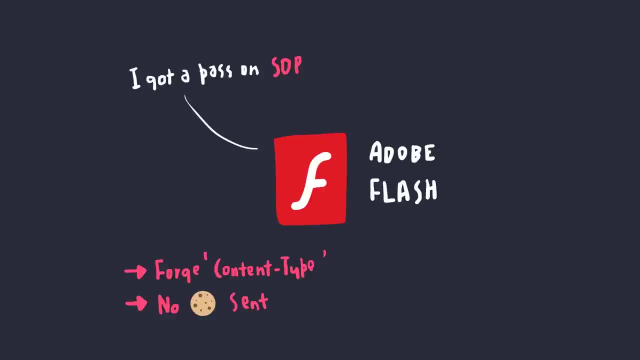 But in order to make this work, We can do a simple redirect, Like a 307 redirect, which holds the headers that are actually being sent, acting like a relay. So the basic idea is that we add a content-type header in the Flash file and all the JSON. 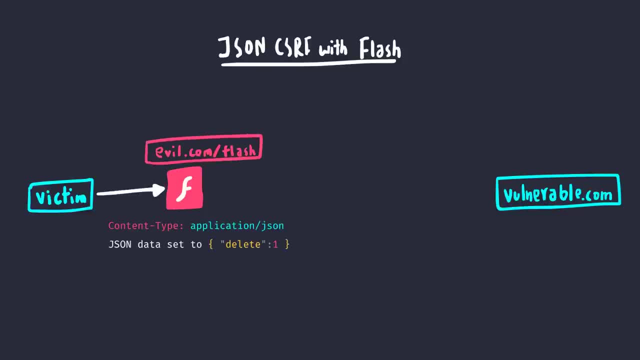 post data that we want to send. We also specify the request endpoint, which is not the vulnerablecom, but instead to our 307 redirect page, which in turn redirects to a vulnerable website. Now We can receive the headers, like content-type header, and also the post JSON data as a string.